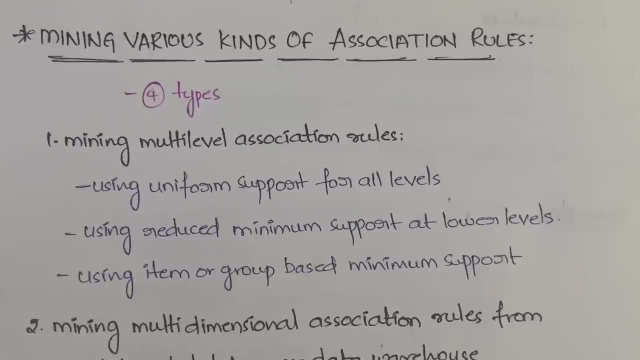 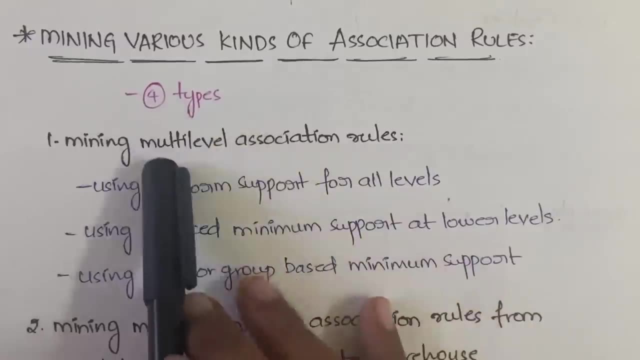 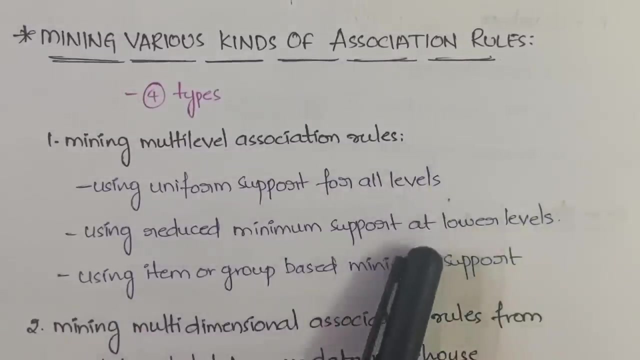 Let us learn now. Okay, First is mining multi-level. So actually we have four types. We are going to discuss about four types. Okay, In the first one only we have subtypes. in the next we don't have any subtypes, Don't worry. Mining multi-level: association rules. See, what do you mean by? 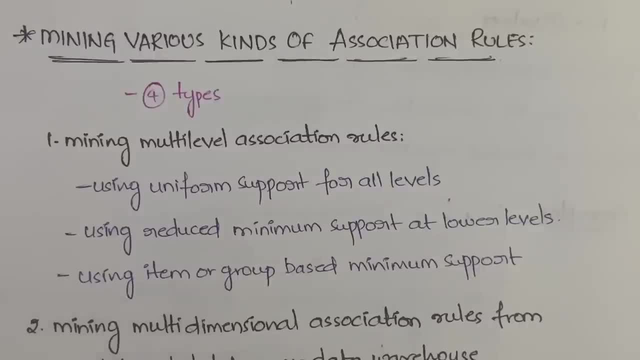 multi-level. So data mining systems have to be- they should be able to mine different levels of association, that they should be able to mine association rules. So data mining systems have to be able to mine different levels of association rules at multiple levels of abstraction. Got it? 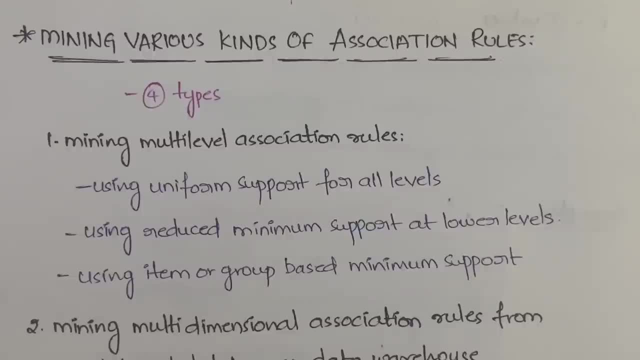 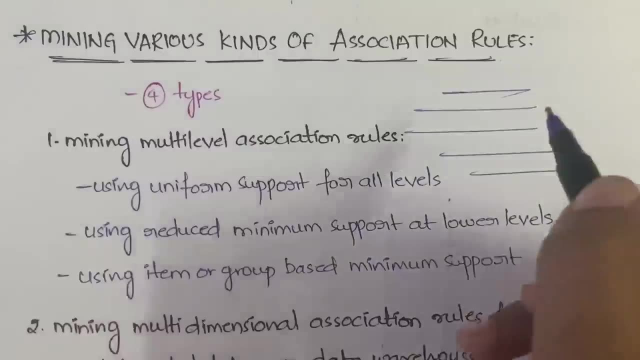 And that too, with the ability to move fastly among different different levels. Suppose you are having five levels of abstraction, then the data mining system which you are using must be able to mine the data at each and every level of abstraction, And it has to be able to move between each and. 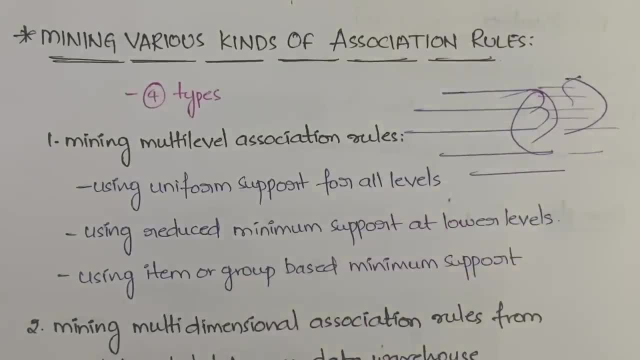 every level easily and fastly Got it. That is what it means. Multi-level association rules is nothing but multiple levels of abstraction. It has to be able to mine And it has to move between different levels easily and quickly. Got it, And you can do that by using. 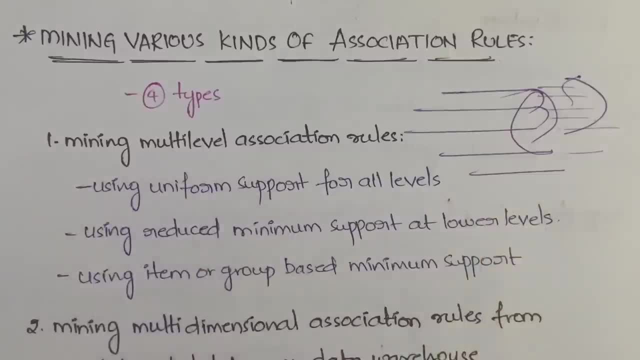 uniform support for all levels, which means that you will be supporting, you'll be setting up a minimum support- 30% or 40% or so- for each and every, for all the levels. Okay, for all the five levels, you'll be setting up a minimum support level that will be same for all the levels. Okay, so you will. 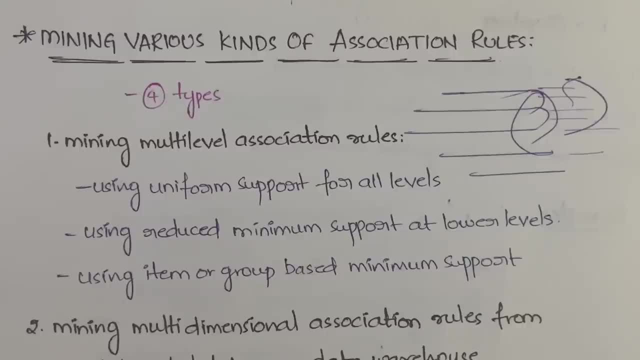 be setting up a minimum support and you will using use any algorithm, like a priori algorithm or any algorithm, and you will be eliminating those- you know, data items whose support is less than the minimum support. Got it Like that. you can do that is first, you have to set up a uniform support to. 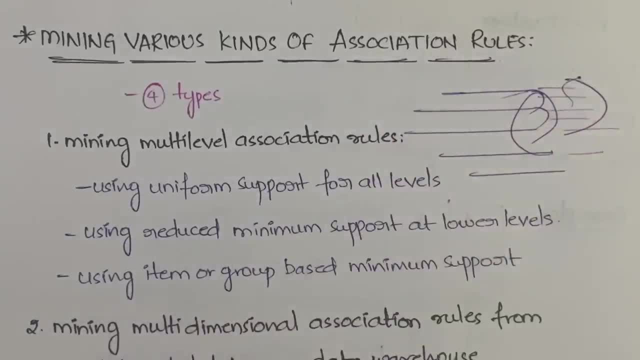 all the levels, which is same for all the levels, And then what you have to do is you have to use any algorithm. by using a priori algorithm, we will be eliminating those data items whose minimum support is less, whose support is less than the value of minimum support, that which we have set. 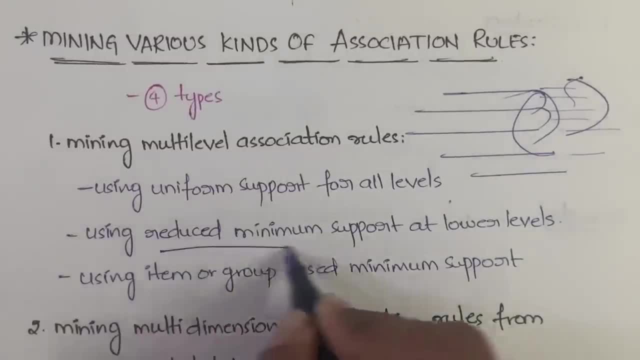 up. Okay. Second step: what you do reduce the minimum support at lower levels. What do you mean? means each level of abstraction will have different minimum support. here we will be set up in different, different minimum support levels for each level, based on the level, or based on the priority, or based on the. 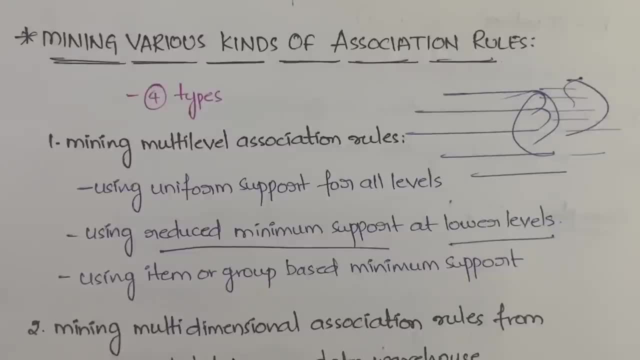 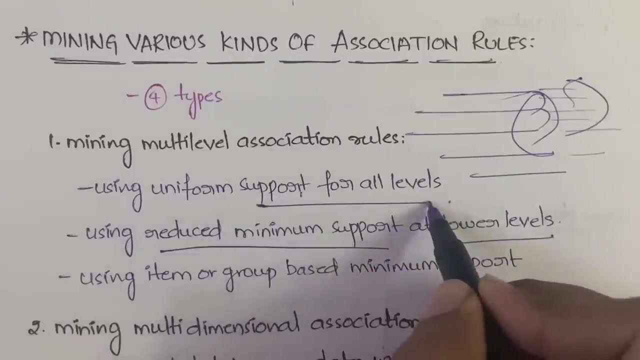 importance, which lower levels will be given. lower minimum support. Okay, And even after giving less amount of minimum support, also, if lower levels are not able to satisfy it, we can remove those lower levels. Okay. next, Here you're using the same support, uniform support, that is. 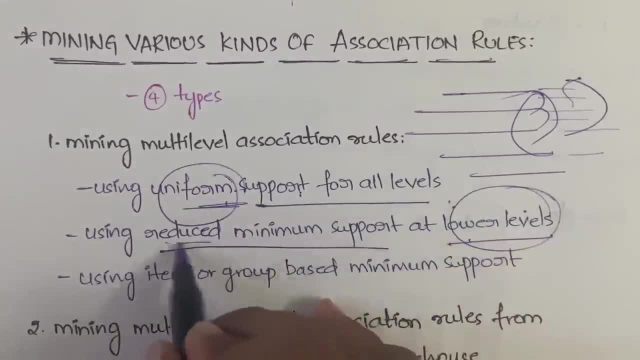 same for all the levels, but here, for lower levels, you will be reducing the minimum support value. That's all using item or group based minimum support. So here what you will do is based on the importance of that item. if that item is very important, you will be giving it less priority, less support or more. 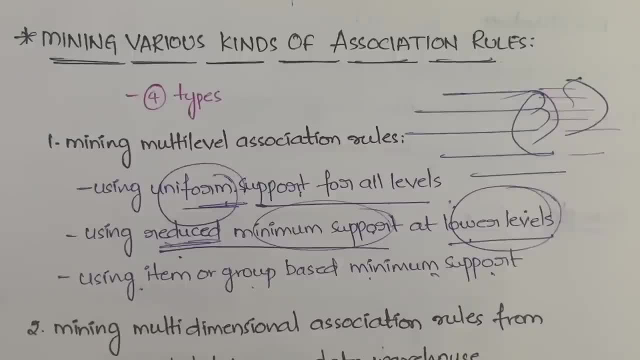 support like that, based on the importance of the item, you will be giving the support and based on that support, you will be eliminating the value. That is about using item or group based minimum support based on the item or importance or the group of items. 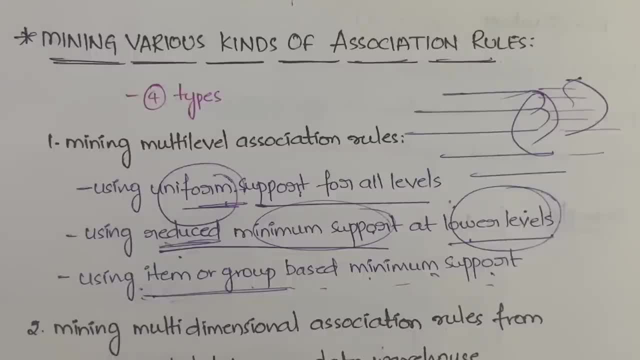 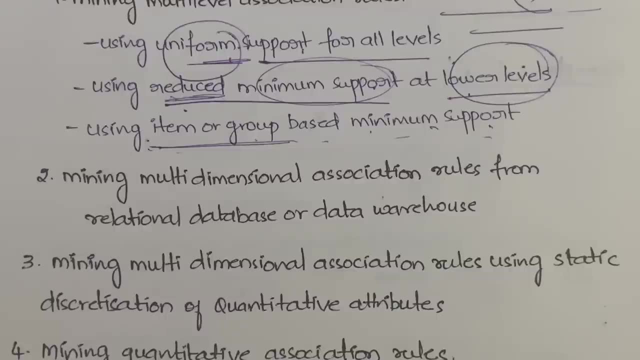 importance. you will be mining the data. Okay, next, mining multidimensional association rules from relational database or data warehouse. that is from relational database, is nothing but our DBMS, that is from tables. data warehouse is nothing, but you know about data. there's large and large amounts of data will be there, And that, too, you. 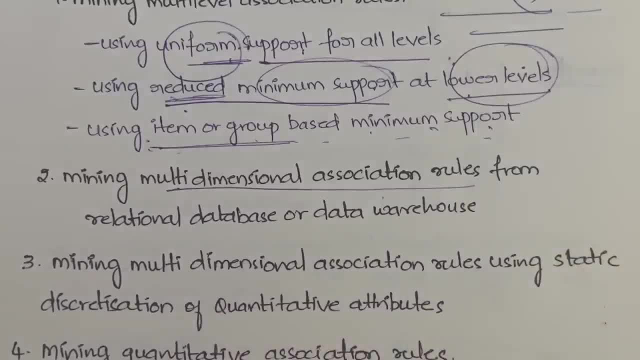 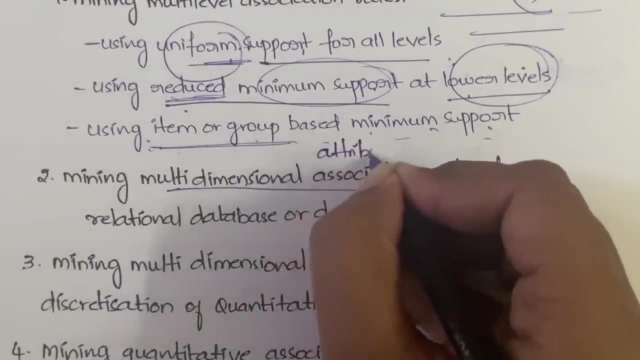 are mining multidimensional association Rules. multidimensional association rules means, see, each attribute will be considered as a, each dimension or each group will be considered as a dimension, So you will have many dimensions got it. when you are mining this kind of data, what you have to do is each attribute. each attribute is considered as a predicate. predicate is nothing but a. 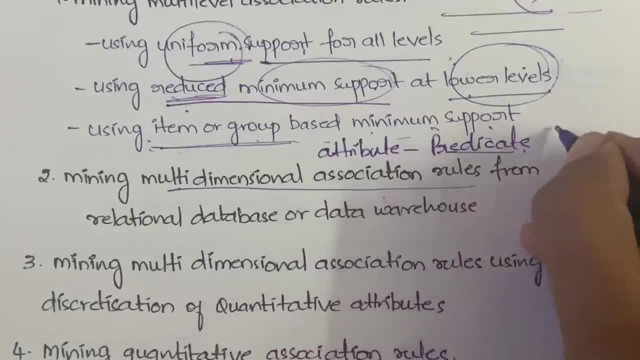 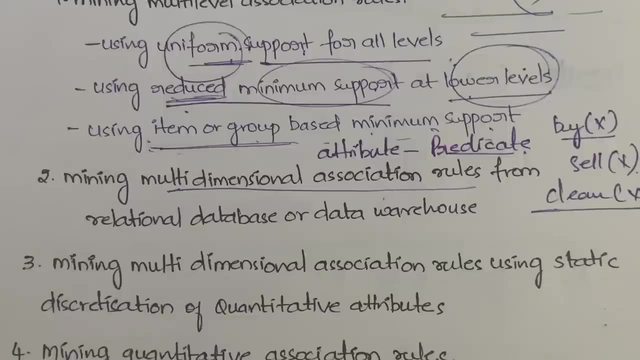 rule. you can say, or you say: like a shopkeeper is buying something, so buy is a predicate. you are selling something, sell is a predicate. you're cleaning something clean is a predicate. so whatever task is being involved, that is a predicate. okay, so what you will be doing is each attribute will be considered as a predicate. 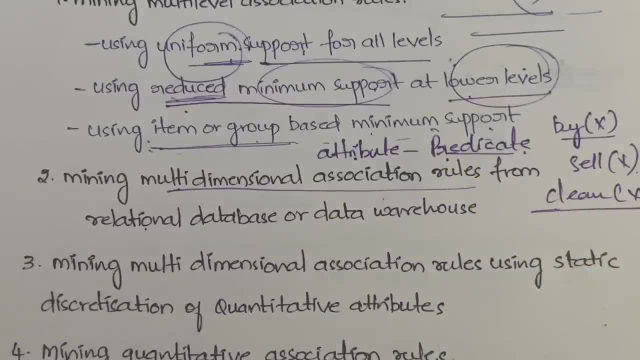 and you will be doing the mining. that's all in rdbms or in data warehouse. that's all. that is what you can write here. each attribute is considered as a predicate and for predicate you can write this example and then data is mined, got it next. mining: multi-dimensional. 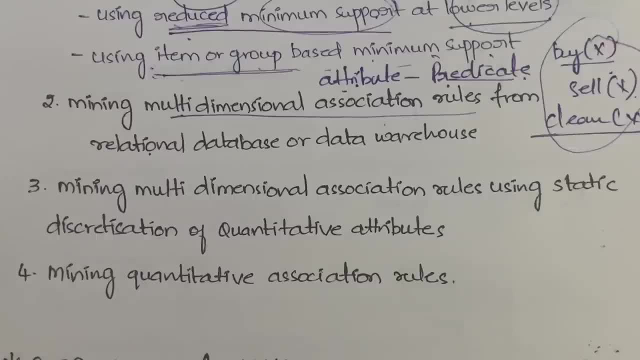 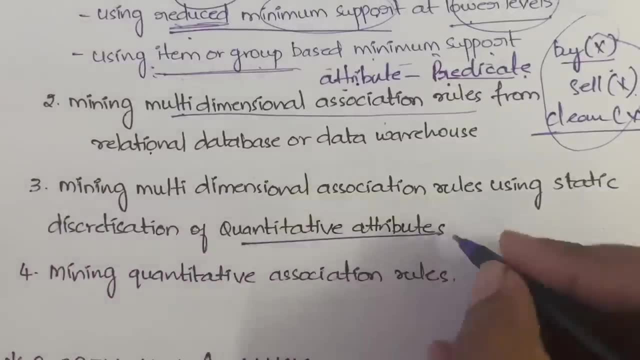 association rules using, starting this, static discretization of quantitative attributes. so first let us go in the reverse way: quantitative attributes is nothing but numerical attributes. okay, so for numerical attributes, you will be using the static discretization. static discretization is nothing, but you will be dividing it into. 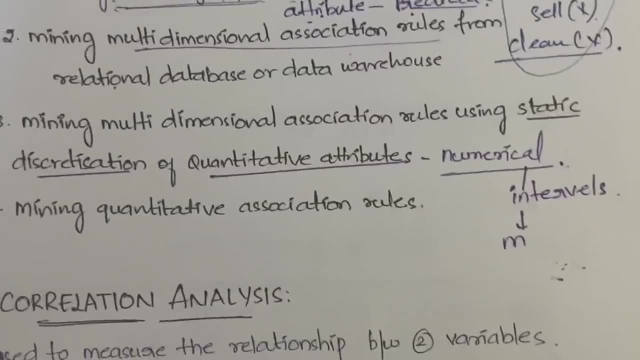 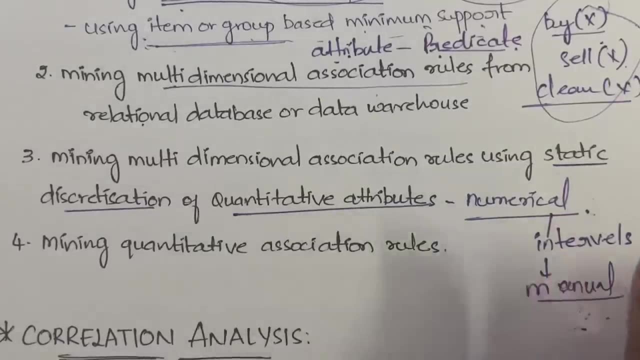 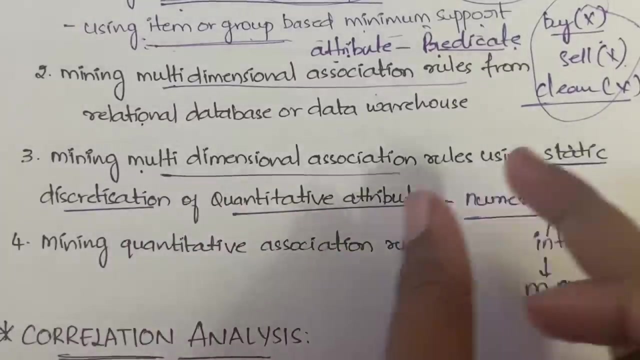 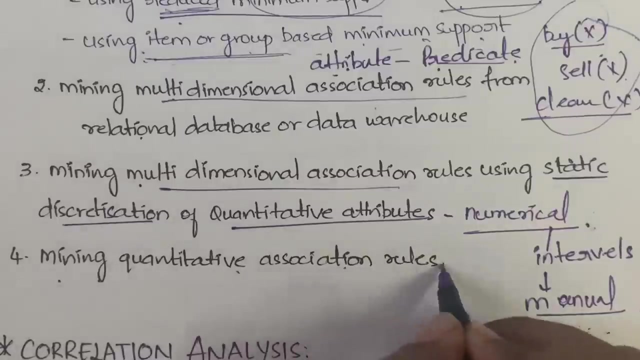 intervals. static is nothing, but manually, on your own, according to our comfortable comfort, we will be dividing. okay, so you will be dividing it into multi-dimensional association. rules are divided into intervals by using static methods, that is, manually we will be doing. next is a fourth one, mining quantitative association rules by dynamic discretization. so same as 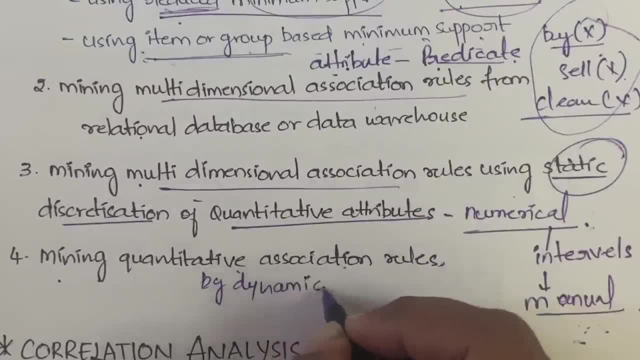 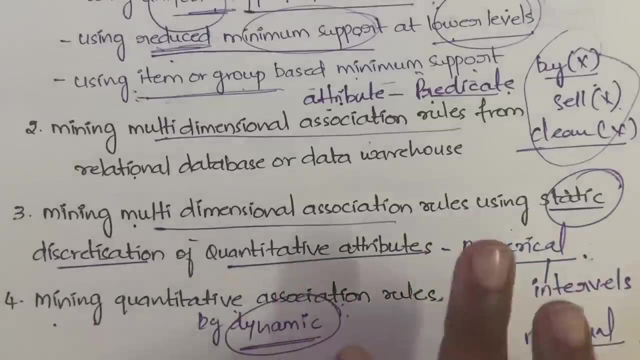 above, but instead of static you will have dynamic. got it dynamic in the sense according to the requirement the computer itself or the system itself will do. we need not manually do anything. okay, this is more efficient when compared to the above one, and this is more efficient in case of large data sets. this will not work in case of large data sets only. 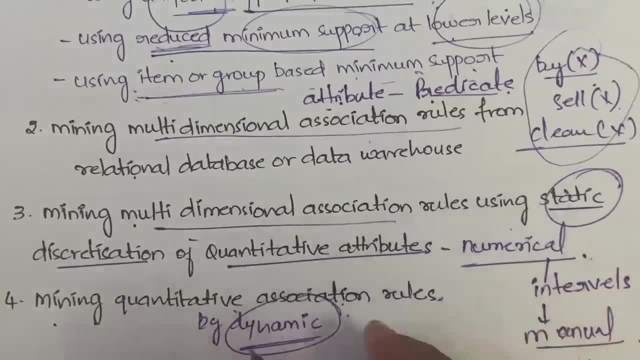 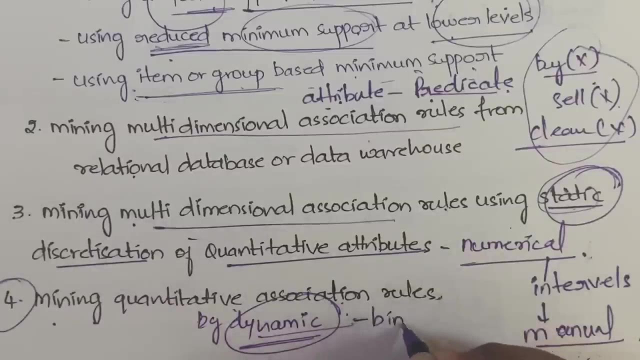 for small data sets, the third one will work. that is the static one. the fourth one is also same as the third, but only difference is, instead of static, you will be doing it dynamically. that's all nothing new. got it now here. this fourth one, that is the dynamic discretization you will be doing with the help of binning. 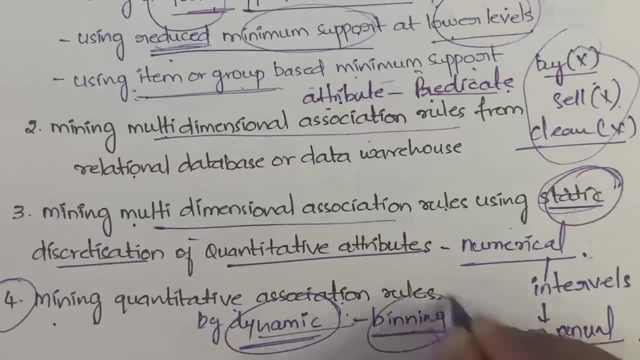 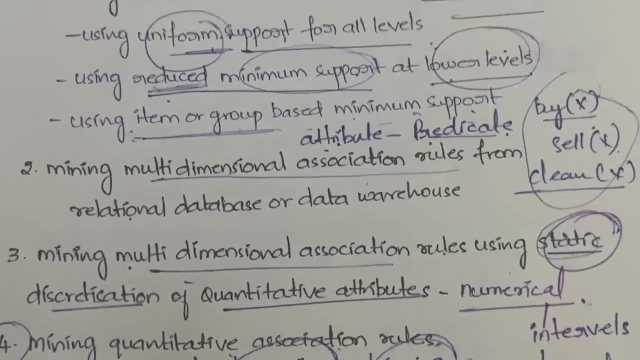 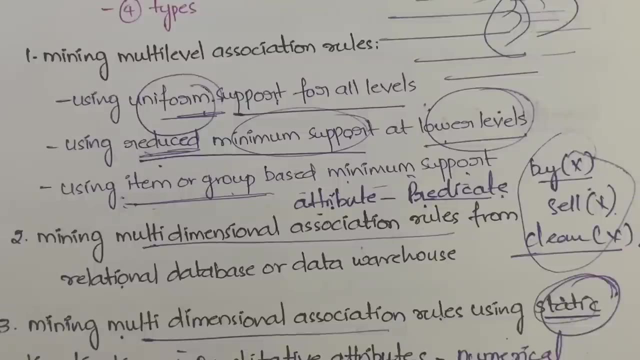 okay, by using the methods like binning and all, you will be doing it. that's all very small, very short video, very simple video. the thing is you have to remember so simple multi-level association rules, multi-dimensional association rules, two types we have. in multi-level we 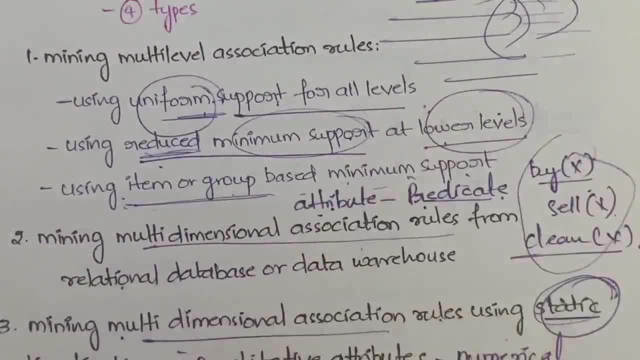 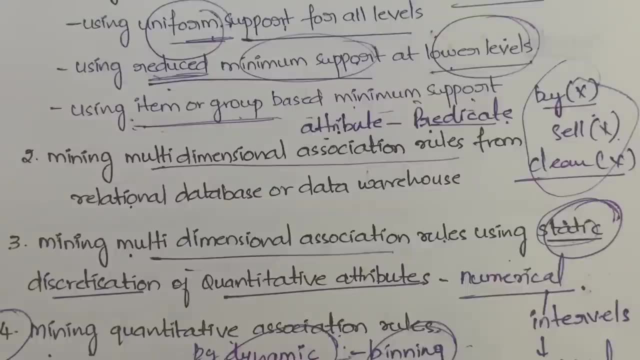 have again three. like you can. we have three solutions for that. in case of multi-level, multi-dimensional, we have three cases. so first one is multi-dimensional association rules for relational databases or data warehouses. second is by using multidimensional association rules for quantitative attributes, in that quantitative attributes also you have.